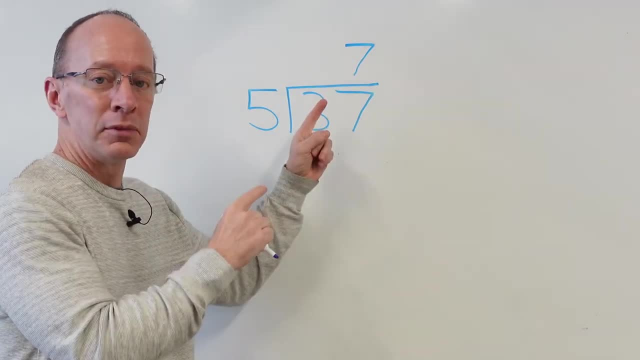 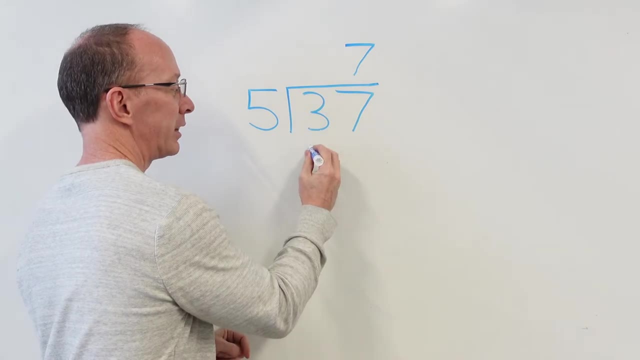 Make sure you line up your numbers correctly and neatly. So now we divided. Now our next step is we need to multiply. So 7 times 5 equals 35. And write that right underneath here. okay, And now our next step is to subtract. 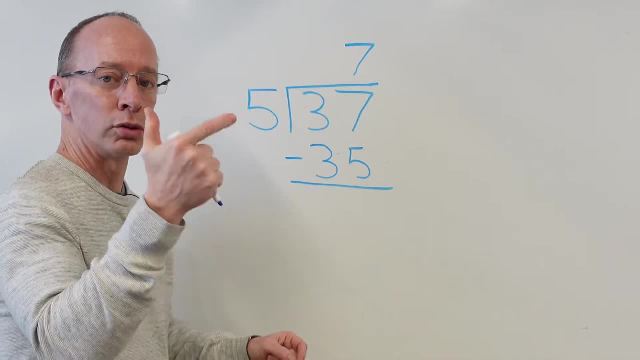 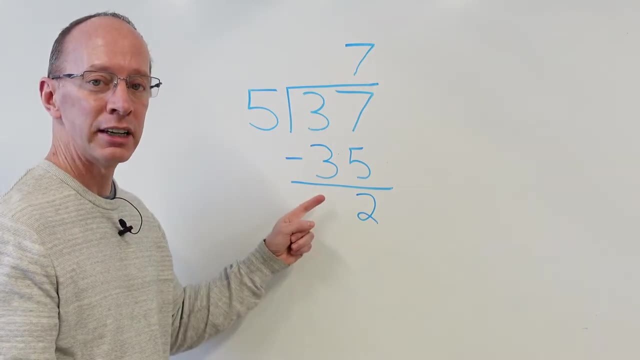 So I go ahead and subtract that 7 minus 5, uno dos. All right, a little Spanish one. two: 7 minus 5 is 2,. all right, 3 minus 3, zero, Zero. 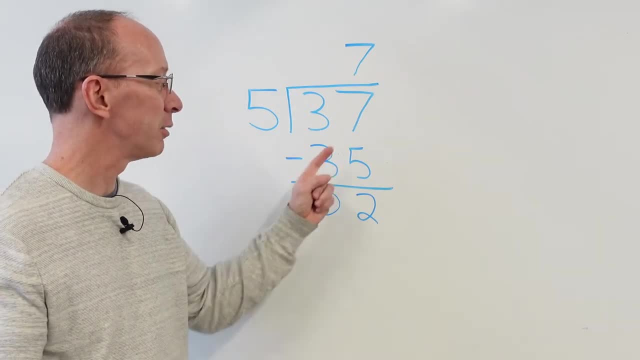 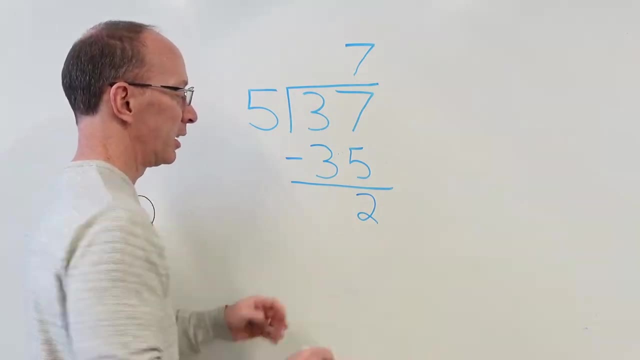 You don't need to put that zero there, because if I were to say, 37 minus 35 equals 0, 2,. no, You don't just just try not to do that, okay, So you just just keep it blank, just 2.. 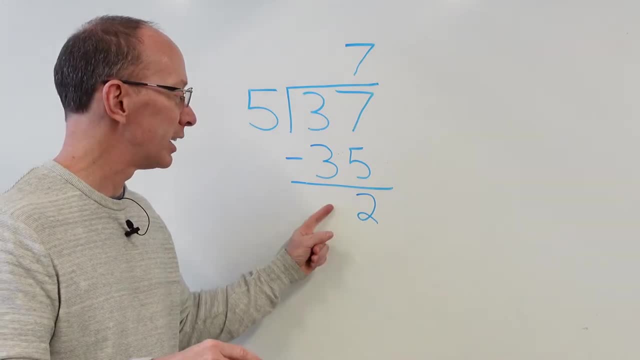 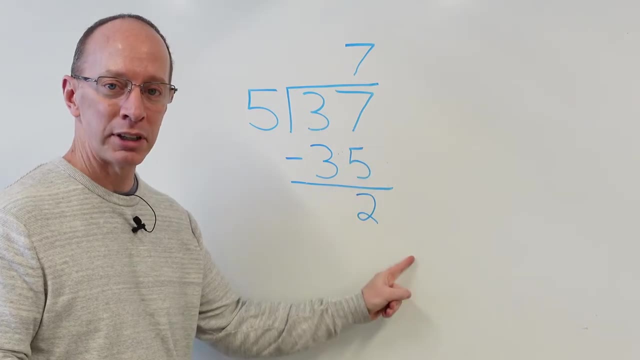 I mean, if you have to, for figuring out, but try to get in the habit of not doing that. So now let's check to see. Can I put 5 into 2? No, Do I have any numbers to drop down? 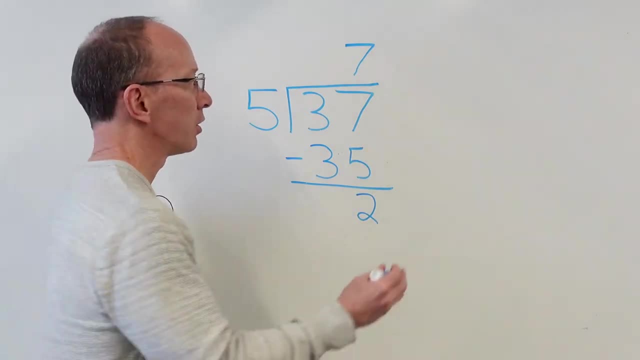 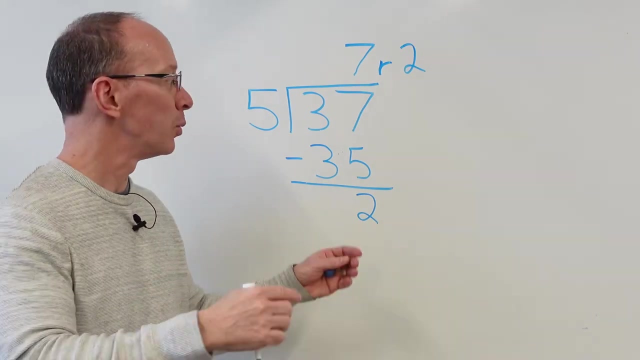 No, This is our remainder, So I put an R right here For remainder 2.. What does this mean? So let's go back to what this problem was about. We had 37 cookies, right? We had to break them into 5 different groups. 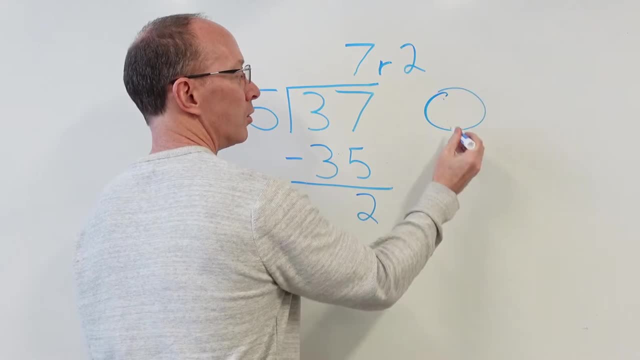 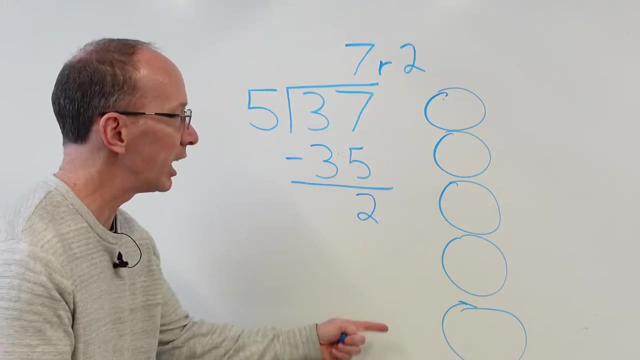 So let's go over here. We're going to make a group, 1 group, 2 groups, 3 groups, 4 groups, 5 groups All the way down here. okay, I got 5 groups. In each of those groups I can put 7 cookies. 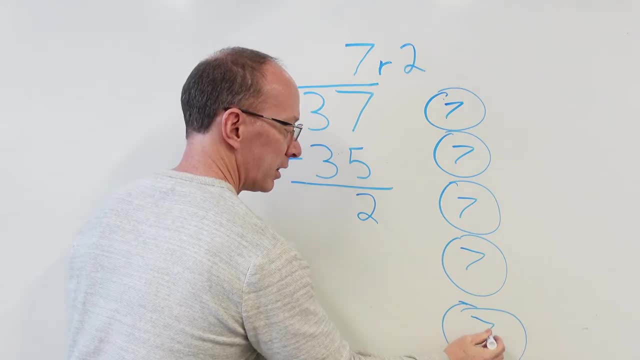 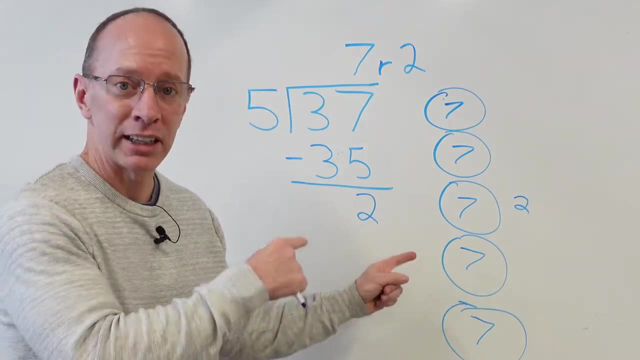 7 here, 7 there, 7 here, 7 there, 7 there, 7 there. okay, And then I have a remainder of 2 cookies that are left over. If you don't mind, I'll take those 2 cookies and then give the rest of the cookies to your friends. 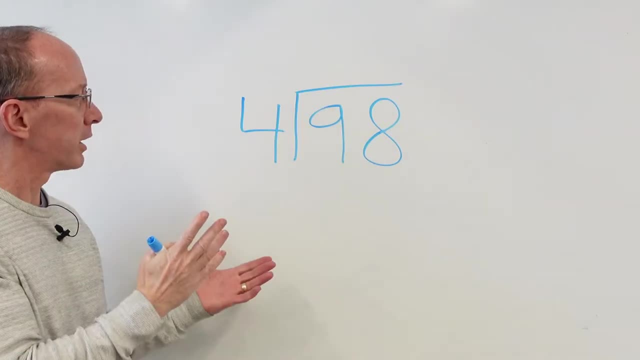 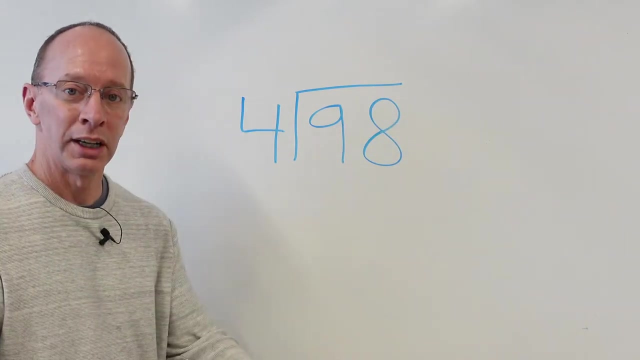 Hey, are you ready to do one more problem? Yeah, let's do it. Yeah, Okay, here we go. We got 98 divided by 4.. Remember, we got to take 98, break it into groups of 4, all right. 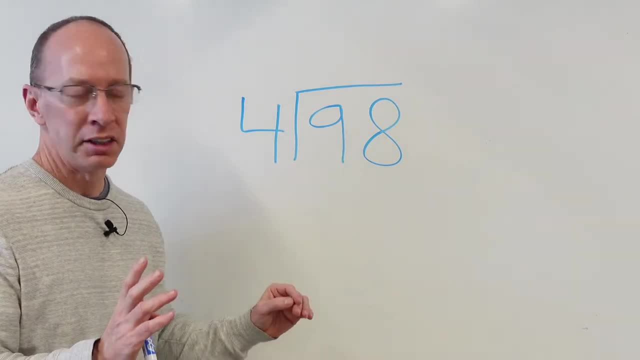 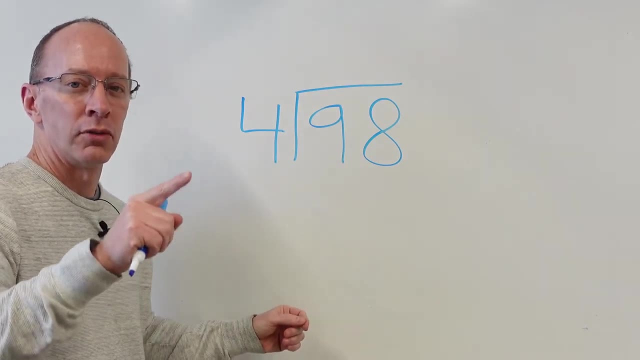 So let's take this slowly, carefully, like a math ninja. First of all, can I put 4 in a 9?? Sure you can. How many times? 4 times 1 is 4.. 4 times 2 is 8.. 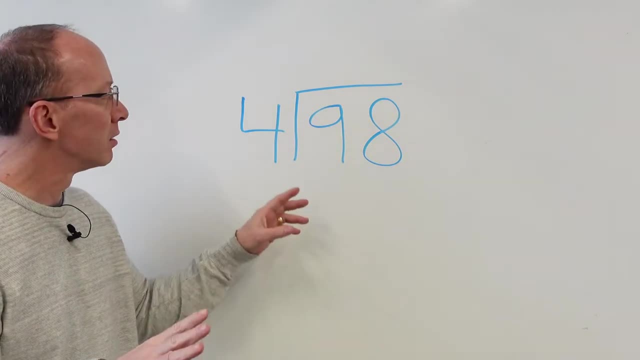 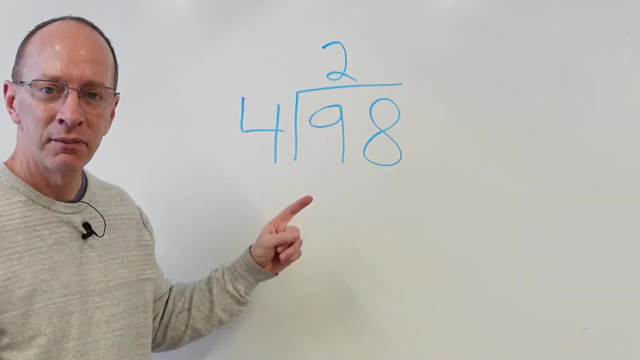 4 times 3 is 12.. Whoa, bring it down, bring it down. bring it down Just 4 times 2.. So I put the 2 right here. okay, Put the 2 right there. I divide it. 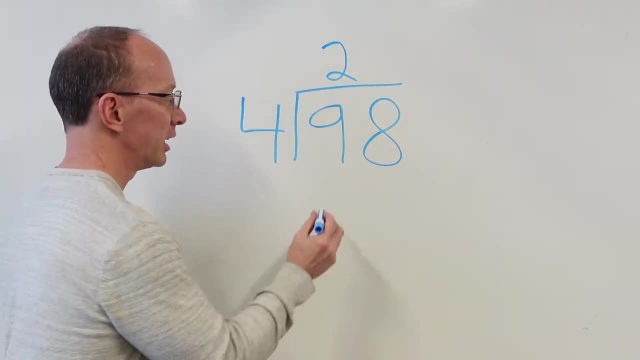 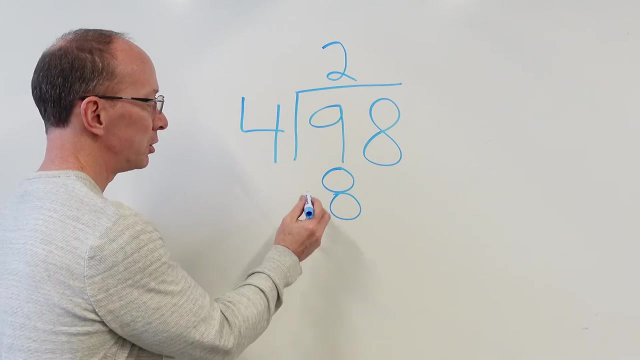 Now I'm going to multiply 2 times 4. is you got it? 8.. 8,, don't be late. okay, Now our next step is 2.. Subtract 9 minus 8, 1, right here. 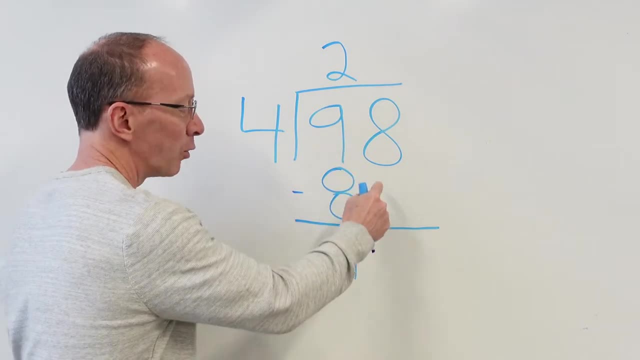 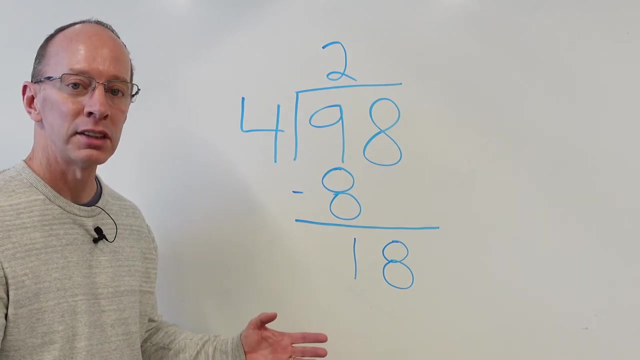 Our next step: bring it down, bring it down. Bring that 8 right down there, okay. Woo drops right down here, okay. Now we start the whole process over. How many times can I put 4 into 18?? 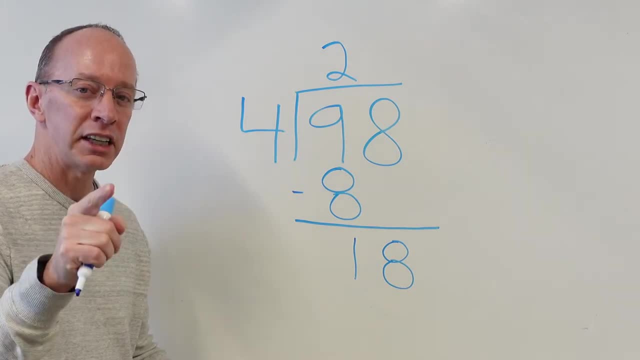 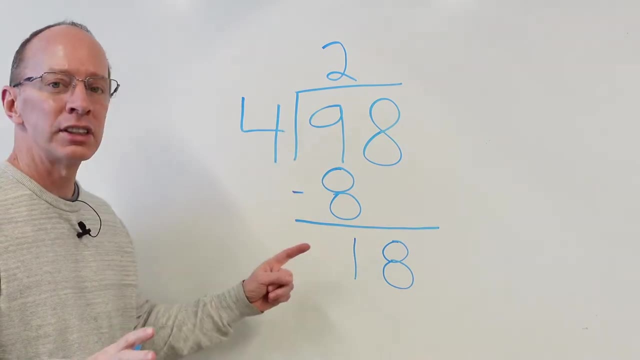 4 times 3 is 12.. 4 times 4 is 16.. 4 times 5 is 20.. Whoa, too high, Bring it down, All right. All right, 4 times 4, we'll stick with that. one is 16.. 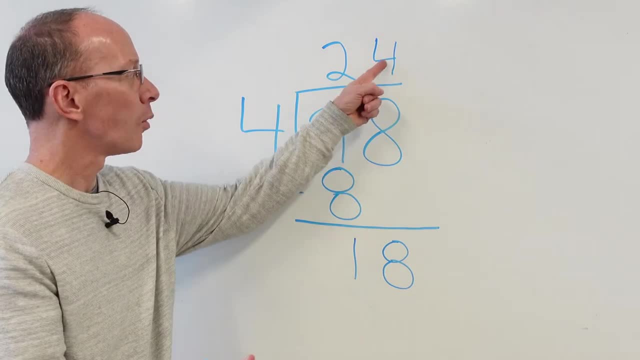 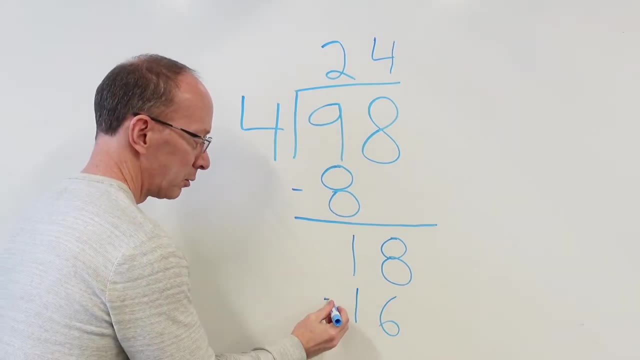 So I put the 4 right here. okay, 4 times 4 equals 16.. And just like what we did here, we subtract. Put a little subtraction sign there, All right, Remember, you subtract the 1's first. 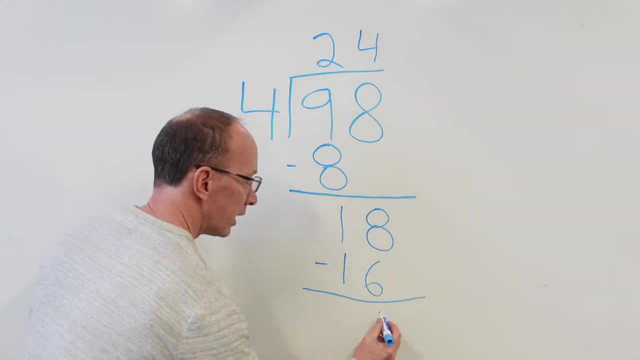 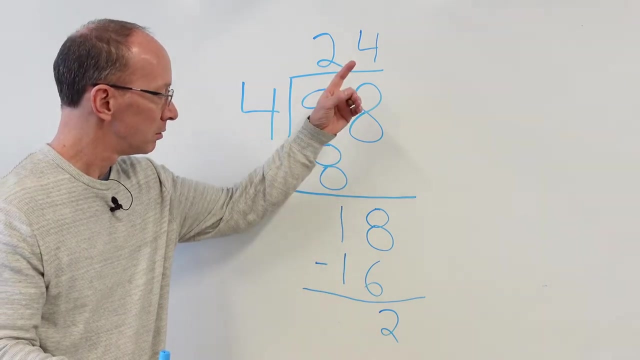 8 minus 6, 1, 2, 1, 2.. All right, put the 2 right here: 1 minus 1,. zip: 0, nothing. Okay, Now our next step. Can we put 4 into 2?? 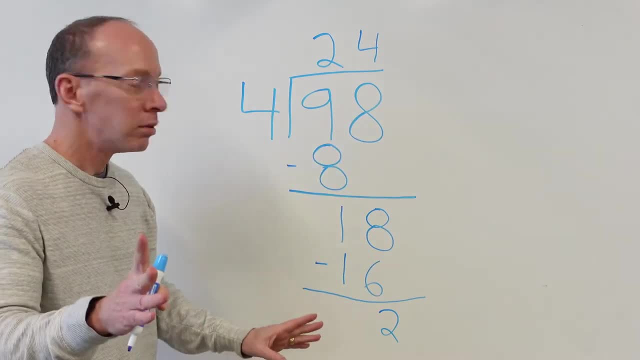 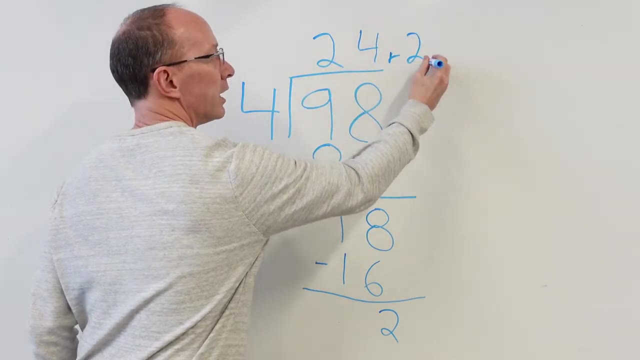 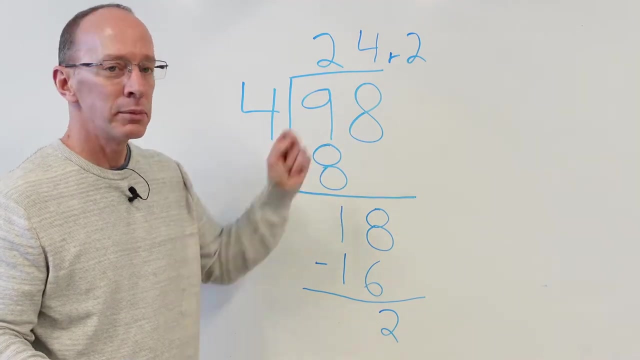 No, Do we have anything to drop down? No, That is our remainder. Bring that all up here. put an R here, put the 2 right there, Remainder 2, all right. So in 4 groups we're going to put 24 in each of those groups with a remainder 2.. 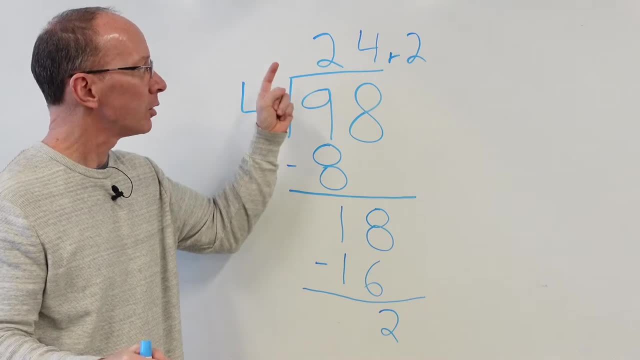 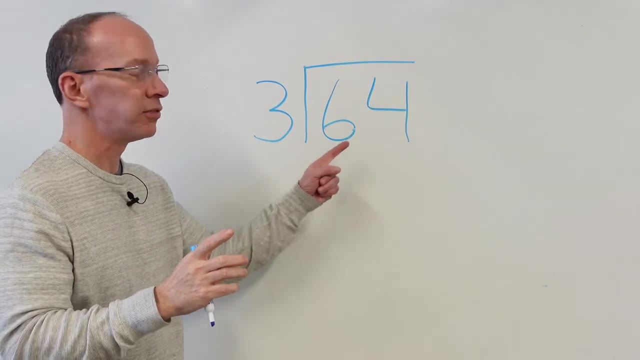 So 98 divided by 4 equals 24 remainder 2.. Ready to do another one? Yeah, let's do it. Yeah, All right, Let's do it. Boom, Okay, We have 64 minus 3.. Can you do it by yourself? 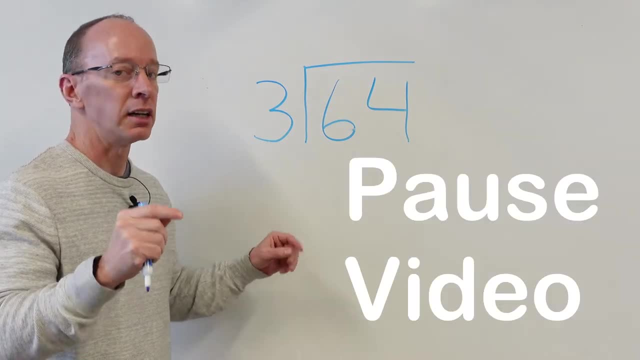 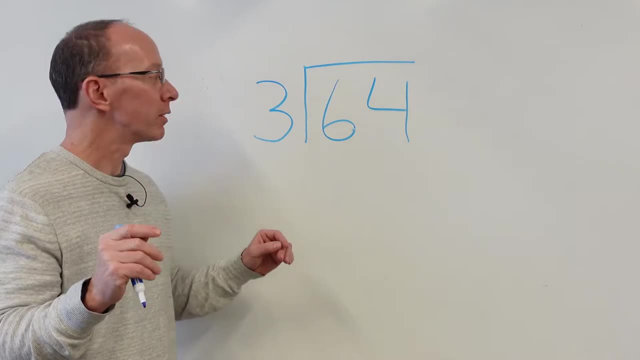 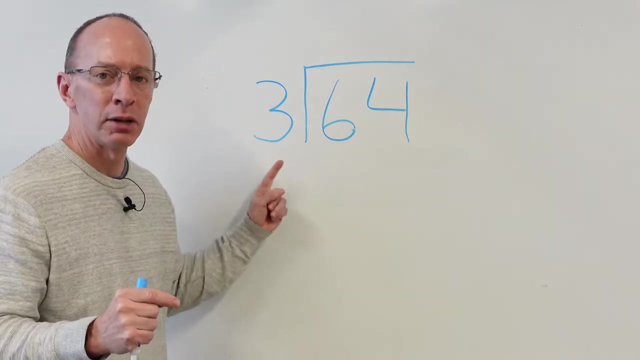 I'll pause the video right here and when you're done, hit play. Okay, Here we go. First of all, 64 divided by 3. Put in your mind what are you trying to do? You're trying to make 3 groups, all right out of this. 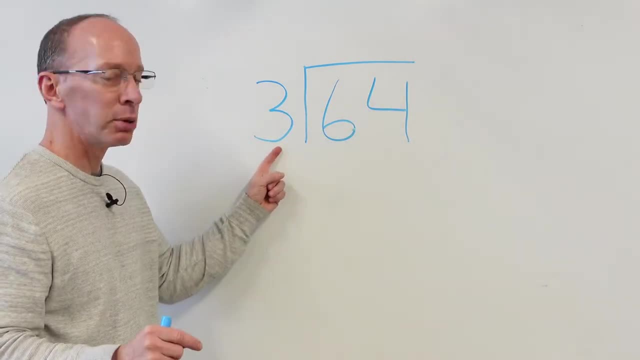 You got to be a math ninja. All right, Here we go. Can I put 3 in this? Can I put 3 in a 6?? Yeah, you can. How many times? 3 times 1 is 3.. 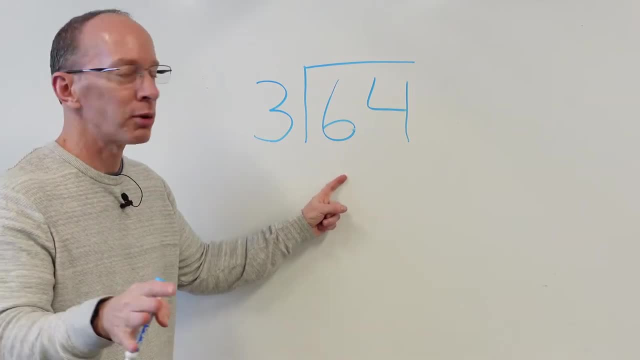 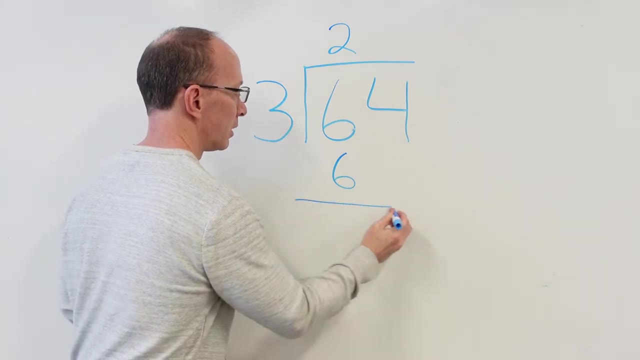 3 times 2 is 6.. Just stop right there. We did it. We hit the mark Jackpot. Yeah, 3 times 2 is 6.. All right, Subtract Nothing. Bring that 4 down right here. 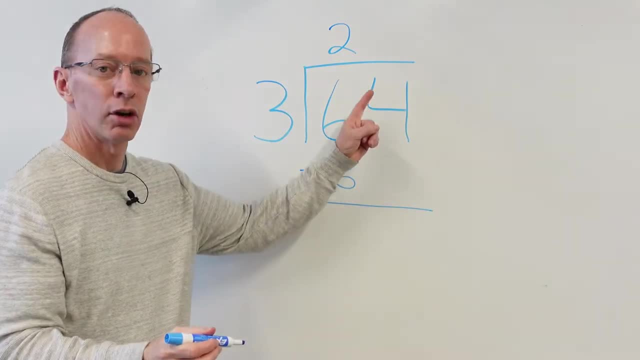 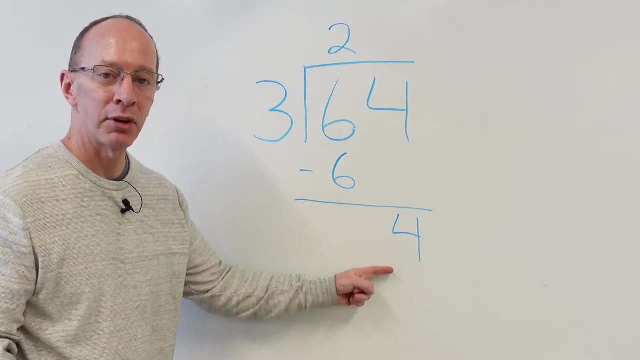 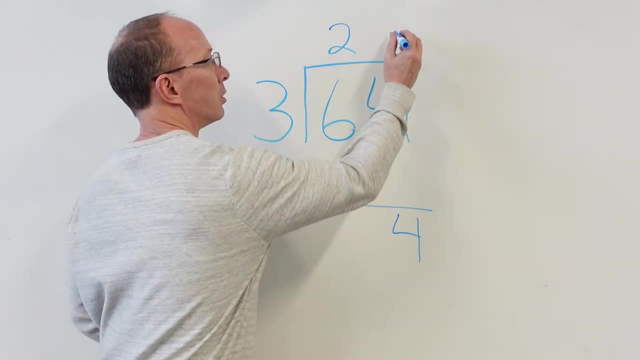 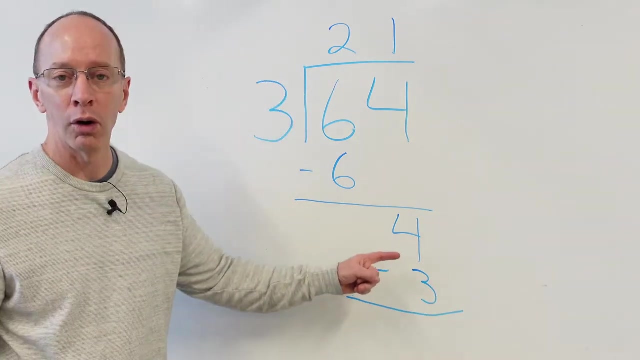 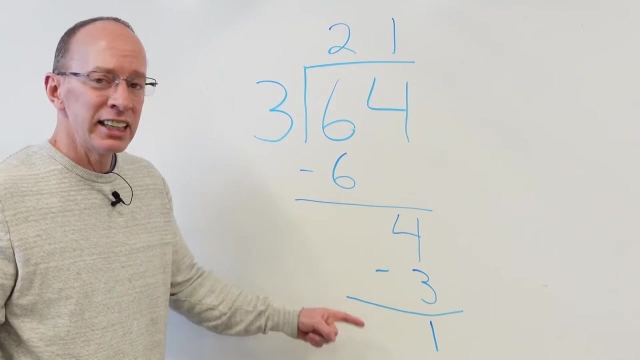 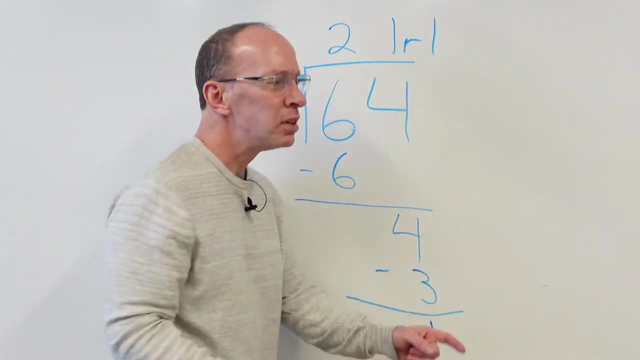 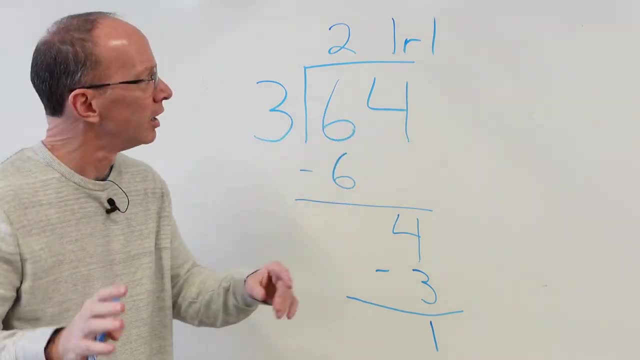 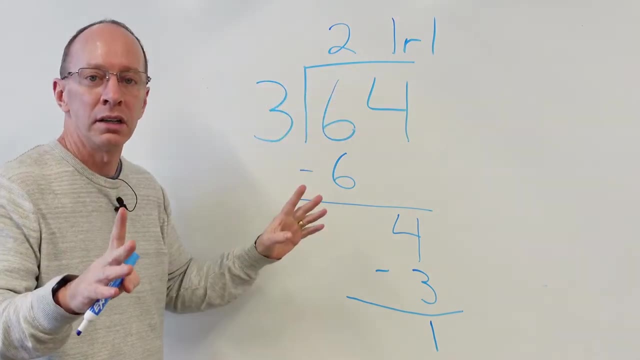 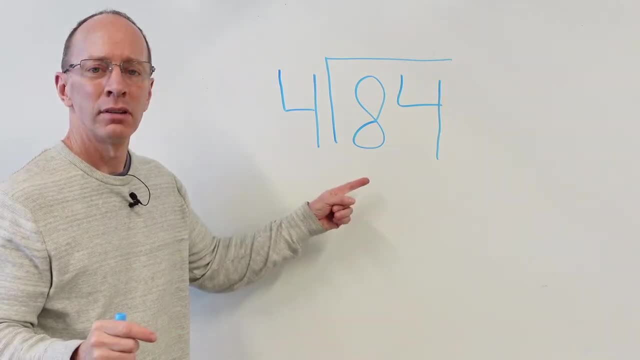 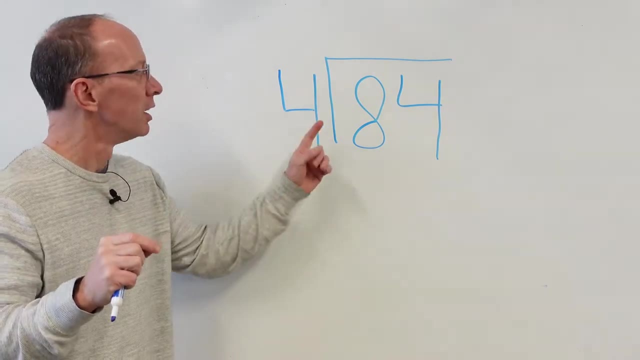 Okay, Here we are Got 84 divided by 4.. All right, Take it Easy: cheesy lemon, squeezy, little by little, baby steps. All right, How many times can I put 4 into 8?? 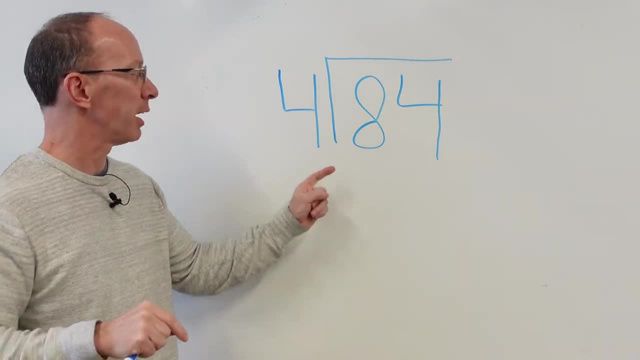 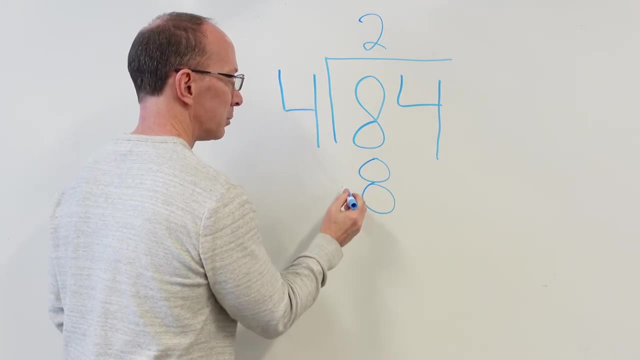 4 times 1 is 4.. 4 times 2 is 8.. Boom, Jackpot. You hit it again. Put the 2 right here. 2 times 4 is 8.. All right, Subtract it, Nothing goes there. 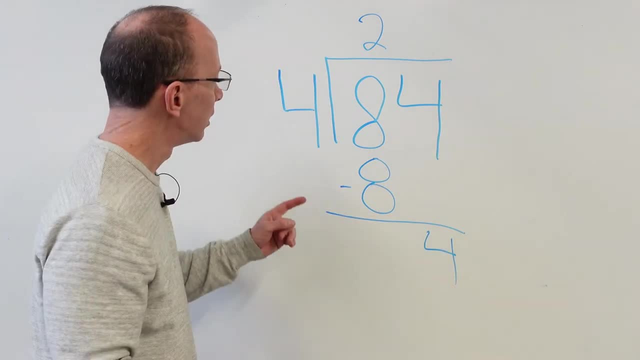 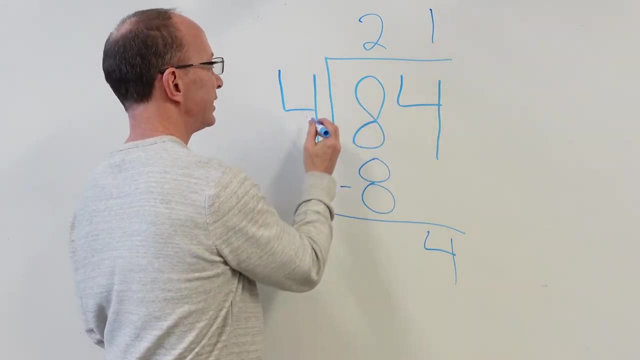 Bring it down. Bring it down. How many times can I put 4 into 4?? 1. Put 4 right in there, All right. 1 times 4 equals 4.. Subtract it 0.. 0.. 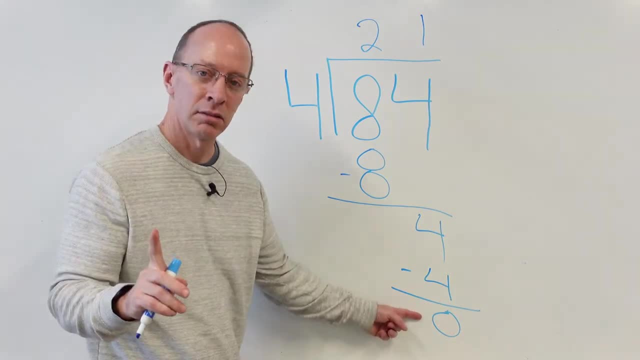 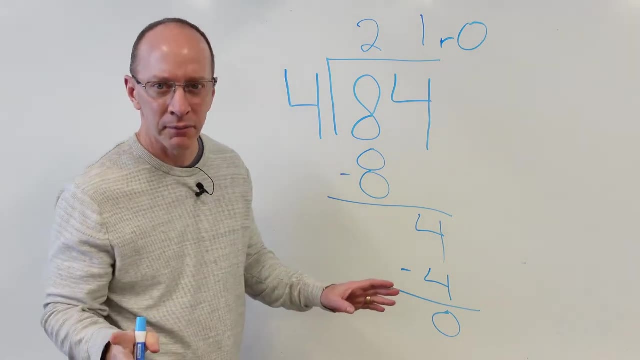 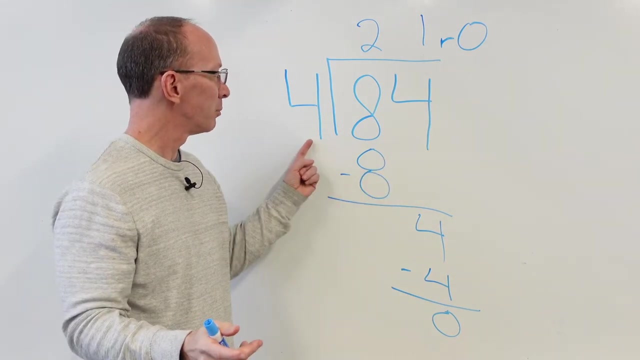 Whoa, Now wait a second. here I've got a 0.. Do I write a remainder 0 right here? Think about it, That's nothing. There's nothing remaining. 84 divided by 4 equals 21, with nothing remaining.